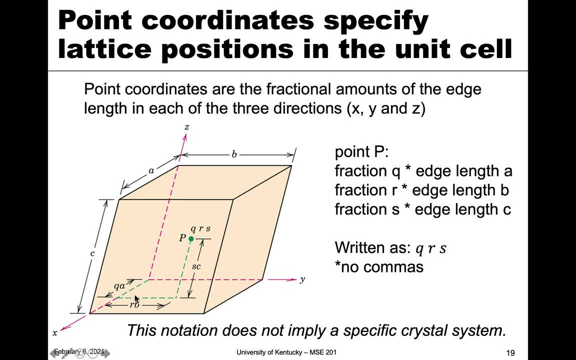 So that's along the- excuse me, along the x-axis. So q is the amount, the fraction of a, and then we have a fractional amount along the y-axis, which is b- the edge length is b- and then the fractional amount along the c-axis, where, or the z-axis, where c is the edge length. 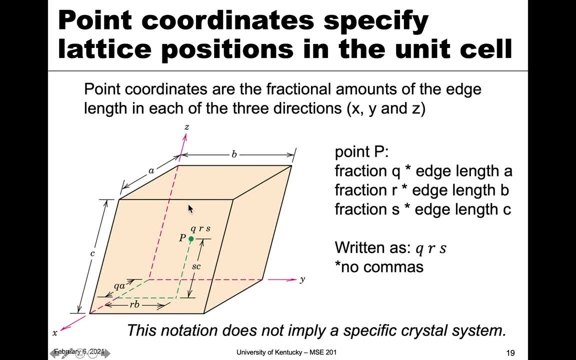 So we have fractional amounts- q, r and s- which define this point, And so it's written. if we want to kind of label point p, we call it q, r, s, and in crystallography, unlike maybe Cartesian coordinates which you've seen before, we don't use commas. 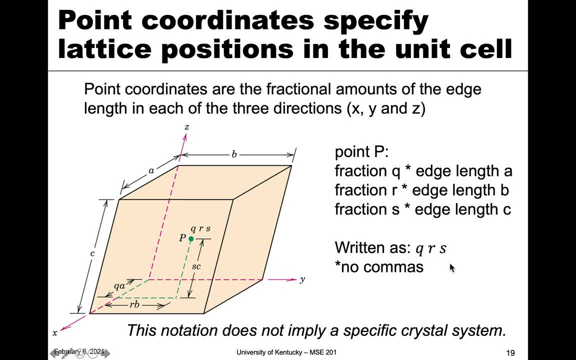 so we just say q, r, s and we don't put commas in between them. So this is the notation that we use for points, for point coordinates, And so, again, the notation doesn't imply a specific crystal system. so this is basically. you can think of this as the triclinic, because it's the most. 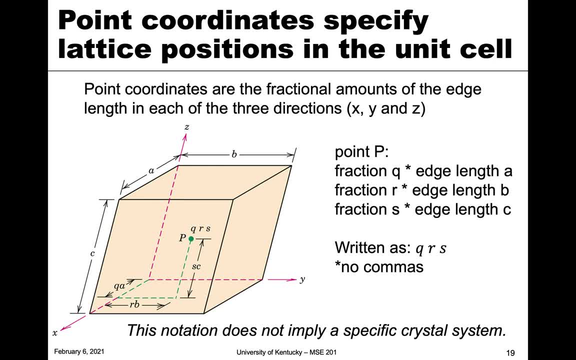 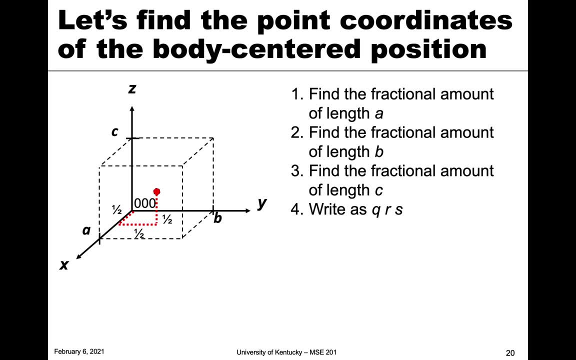 basic structure, but it would work for any other system all right. so i want to kind of show you how we would do this for a given point, right so how we find the point coordinates for a given position. so, for example, the body centered position. let's say we want to label that the body. 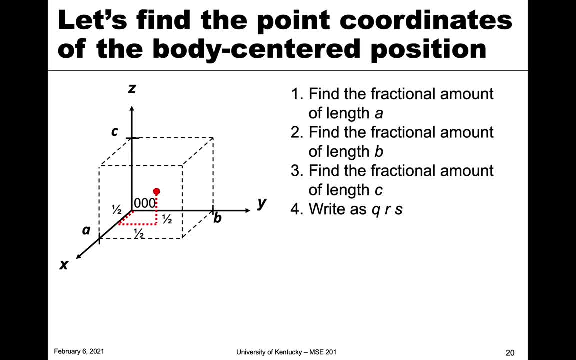 instead of calling body centered, we want to have an actual uh point, uh coordinates for it. so what we do, um, is, you know, we can, kind of excuse me, think of this as starting at the origin, zero, zero, zero, the of this coordinate system, so the, the back left corner of the, the unit cell, and we're 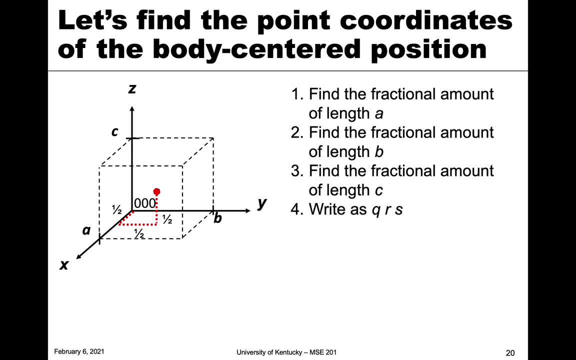 gonna basically find the fractional amounts along each of the lengths. so this is right in the center of the cube and therefore it's going to be in the x direction. it's going to be half of the length a, so the fractional amount there is- sorry, is one half a, and then again, since it's in the center,